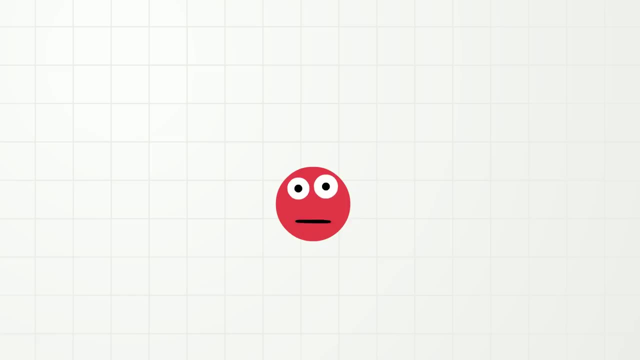 we are going to practice with our hands. Most people have two hands: A left hand and a right hand. Now let's make a pattern: When I say left, raise your left hand high. When I say right, raise your right hand high, And you can say the words with me too Ready, OK, go. 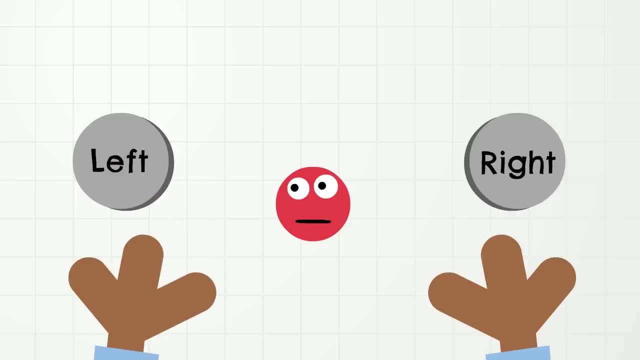 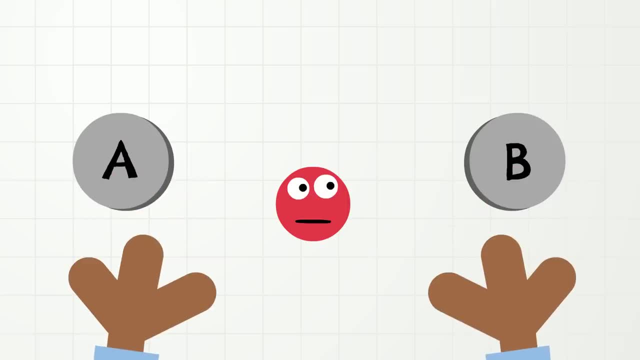 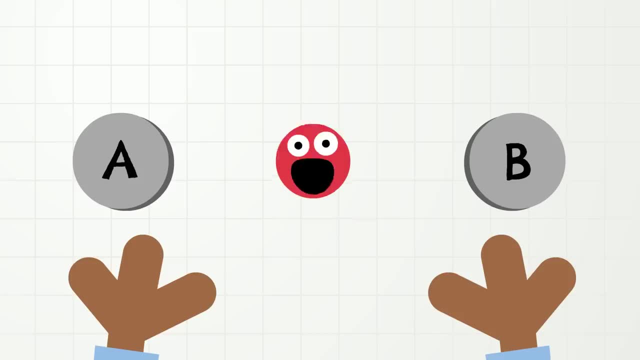 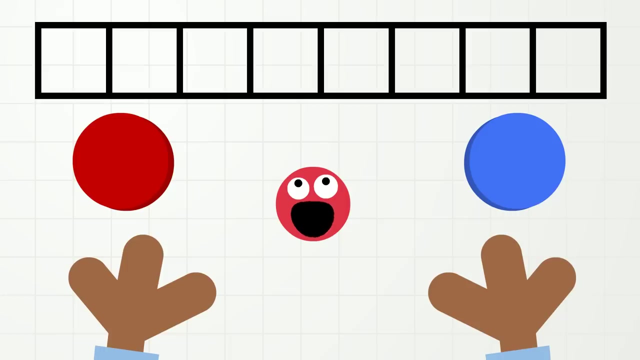 is also called an A-B pattern, Fascinating. OK, now let's make an A-B pattern, but with a color- colors- red and blue- And we will also see what this pattern could look like too. at the same time, Ready. 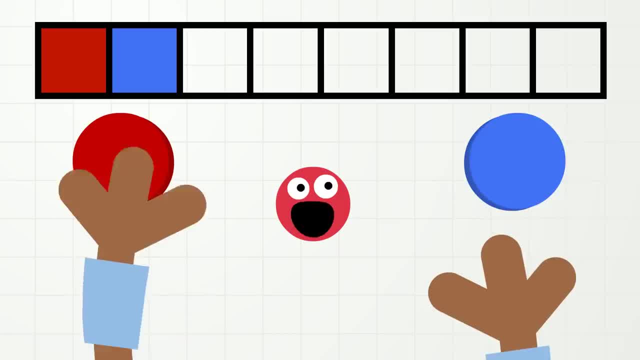 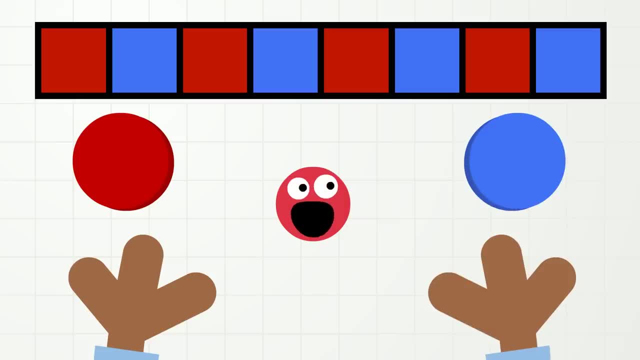 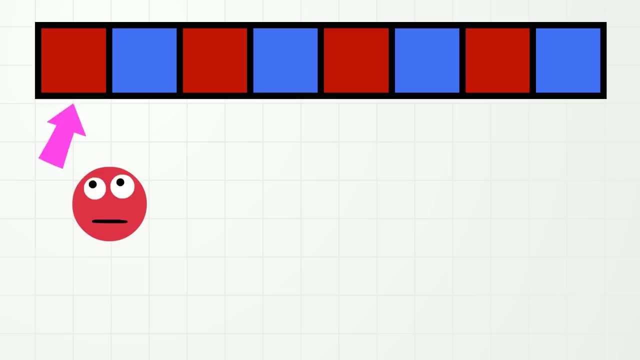 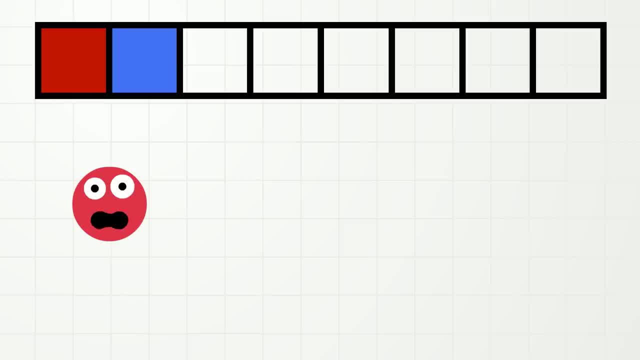 It is not just the red that happens again and again, and it is not just the blue that happens again and again. it is the red and the blue together, And it is this red and blue core that always repeats, repeats, Boop. 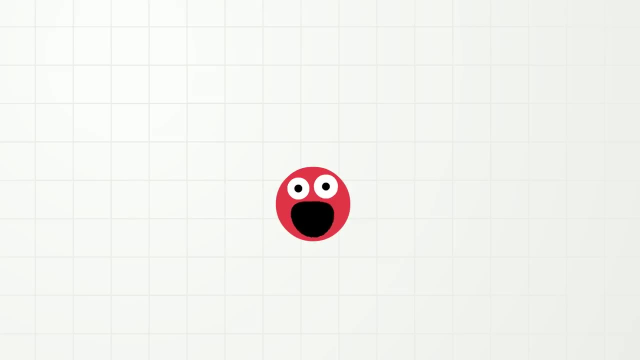 Ok, you've done such a good job. It is now time for a break. Let's take a break outside. Ok, that's enough. Now let's make some more patterns, but this time, instead of two different things that repeat, there will be three different things that repeat. 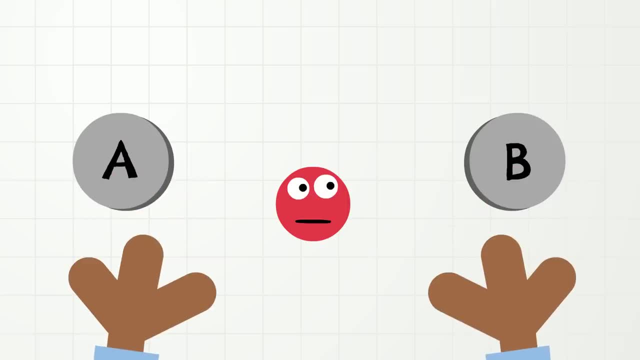 Stir, stir, Michigan music, Just like that. A and B, Oh wow, good job. A and B repeat in the same order. so that was a pattern. And guess what? A pattern that has two things that repeat, like that is also called an A- B pattern- Fascinating. 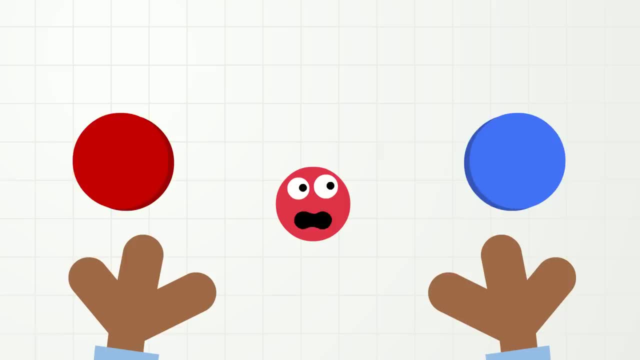 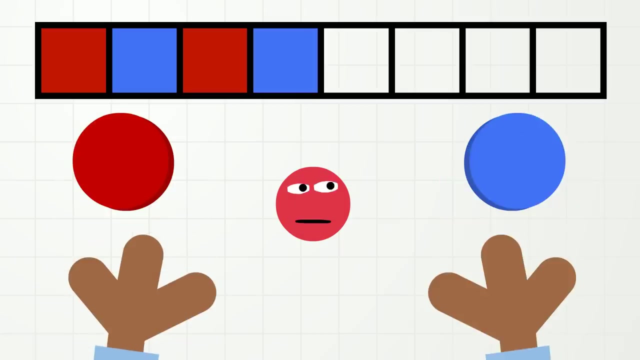 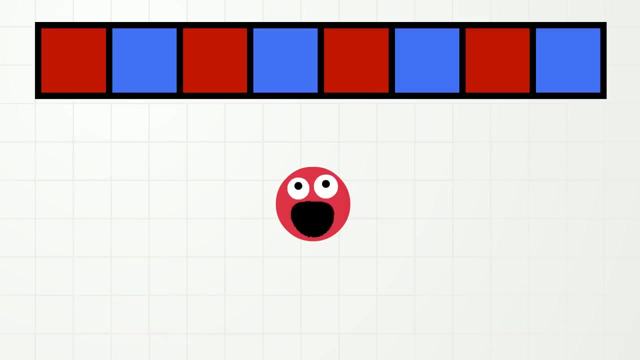 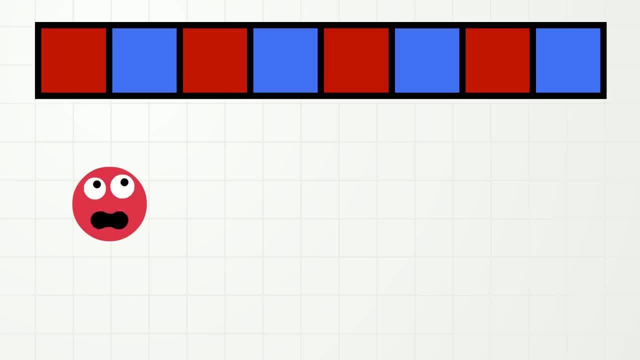 We know that it is a pattern with two things- red and blue- And we can say that this is the core of the pattern. It is not just the red that happens again and again, and it is not just the blue that happens again and again. it is the red and the blue together. 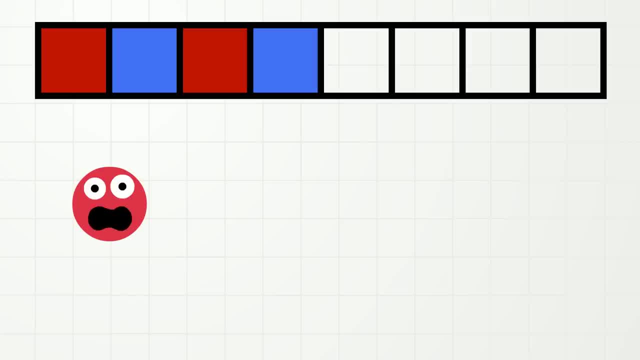 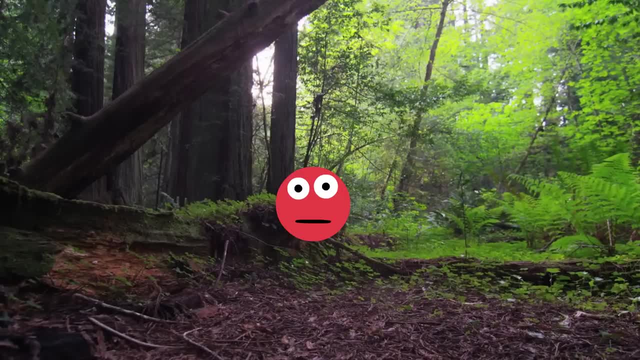 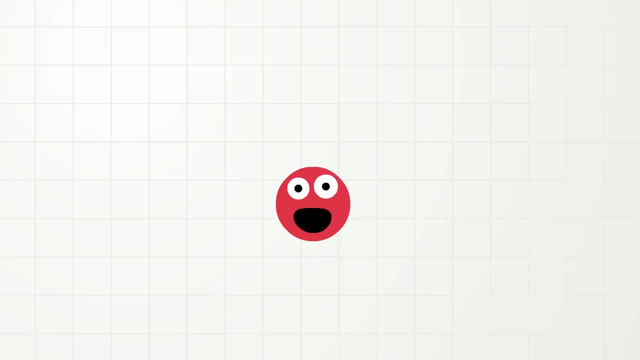 And it is this red and blue core that always repeats, repeats, Boop. Ok, you've done such a good job. It is now time for a break. Let's take a break outside. Ok, that's enough. Now let's make some more patterns, but this time instead of two different things, that. 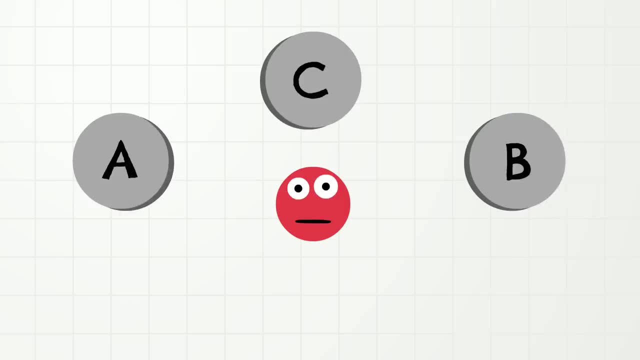 repeat. there will be three different things that repeat, And this is sometimes called an ABC pattern. so let's use those letters Now. instead of the order going left and right, it is going to go left right up. Let's do this together. 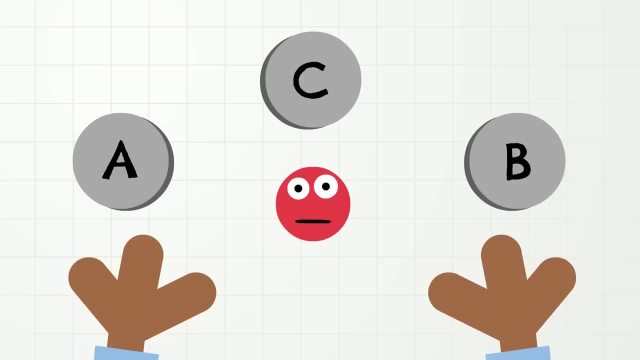 Let's do it with our hands and our voices. Ready, Ok, go A B C. A B C, A B C. Wow, Ok, let's do another three-thing pattern, but this time with something else. 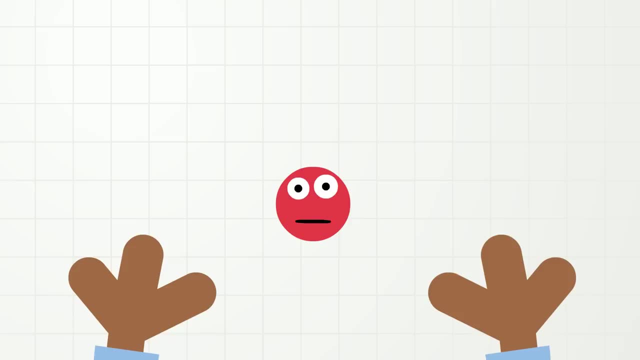 What can we use? Oh, I know How about popcorn: unicorn and mustache Popcorn. unicorn and mustache Popcorn. popcorn and mustache. Popcorn. popcorn and mustache. Popcorn. popcorn and mustache. 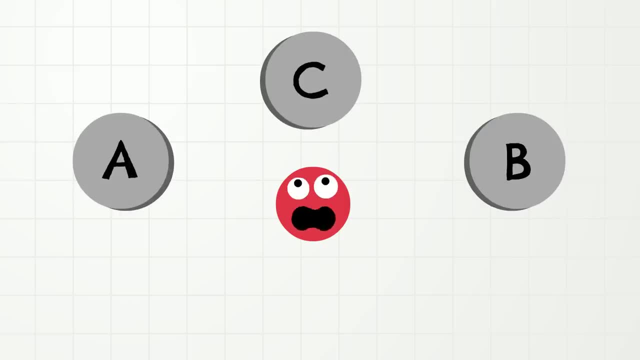 And this is sometimes called an ABC pattern. so let's use those letters Now. instead of the order going left and right, it is going to go left right up. Let's do this together. Let's start with our hands and our voices. 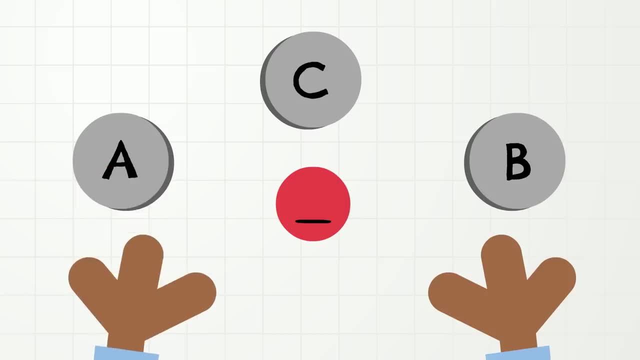 Ready? Ok, go A B C, A B C, A B C. Wow, Ok, Let's do another three thing pattern, but this time with something else. What can we use? Oh, I know. 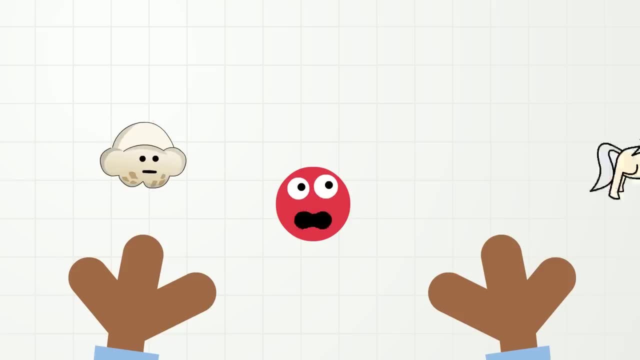 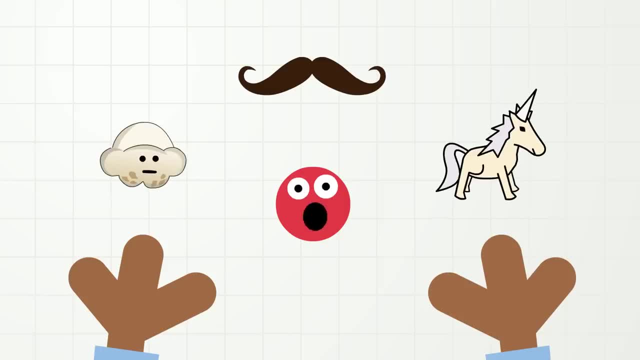 And let's also see what a popcorn, unicorn and mustache pattern would look like. too Ready, Ok go. Popcorn unicorn, mustache, Popcorn, unicorn, mustache, Popcorn, unicorn, mustache. Ok, good job. 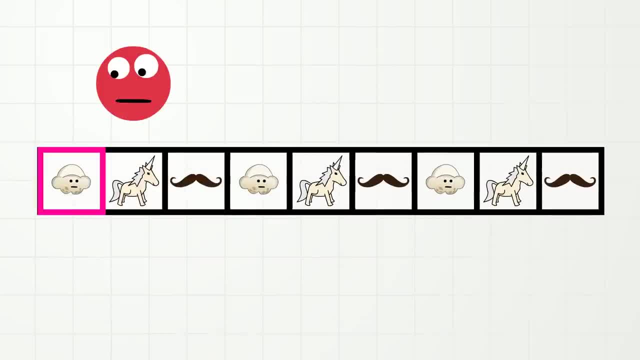 So we know that this is a pattern with three things- popcorn, unicorn, mustache and that- and that this is the core of the pattern, And the core always repeats, Repeats, Boop. And now I have some questions. 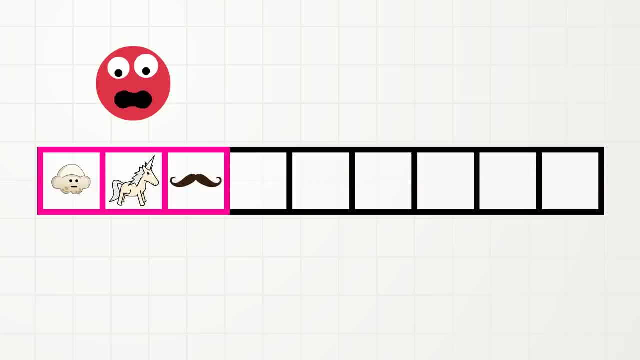 Question number one: Here is the core of the pattern: Popcorn, unicorn, mustache. So what would come next? right here, That's right, It would be popcorn, Yay. And after popcorn, right here, what would come next? 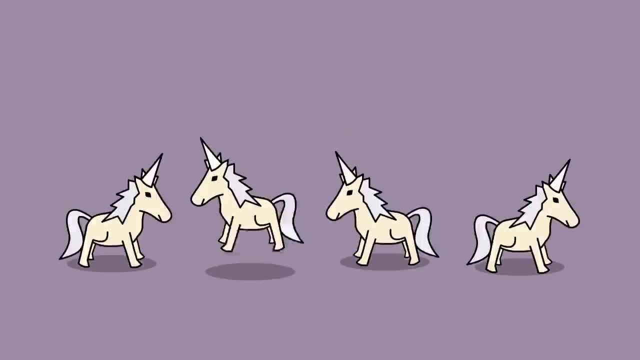 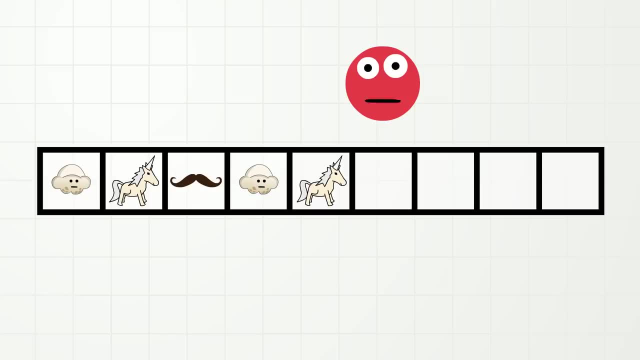 That's right, It would be unicorn, Yay. And after unicorn, what would come next? That's right, It would be mustache- Yay. Question number two: What do you think would happen if the pattern keeps going? Do you think it would stay the same? 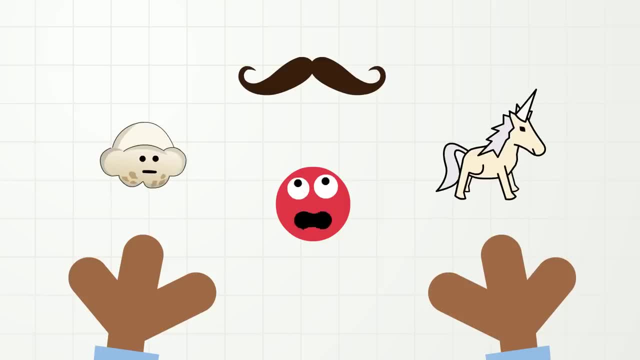 Popcorn, popcorn and mustache. Popcorn, popcorn and mustache. Popcorn, unicorn and mustache. And let's also see what a popcorn, unicorn and mustache pattern would look like. too Ready, Ok, go. 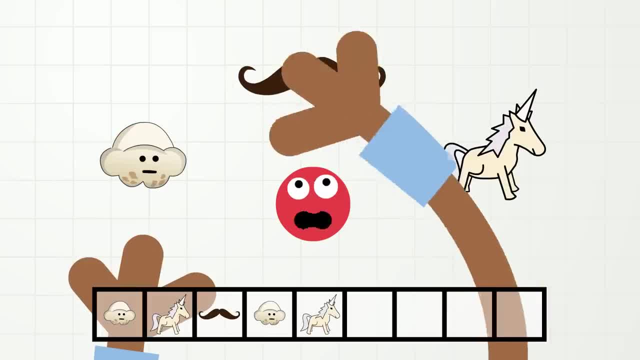 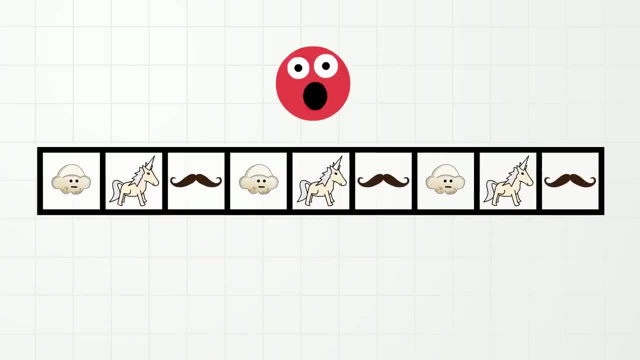 Popcorn- unicorn- mustache. Popcorn, unicorn and mustache. Popcorn, unicorn and mustache. Ok, good job. So we know this is a pattern with three things: Popcorn, unicorn and mustache. 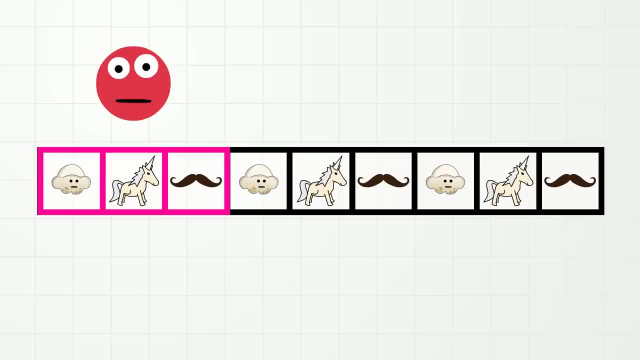 And that this is the… core of the pattern. and the core always repeats, repeats, boop. And now I have some questions. Question number one: Here is the core of the pattern: popcorn, unicorn moustache. So what would come next right here? 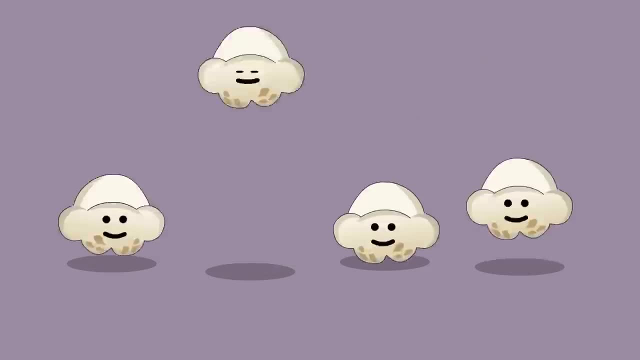 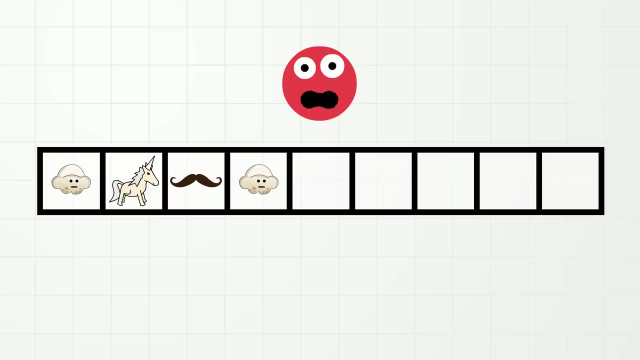 That's right, it would be popcorn, yay. And after popcorn, right here, what would come next? That's right, it would be unicorn, yay. And after unicorn, what would come next? That's right, it would be moustache, yay. 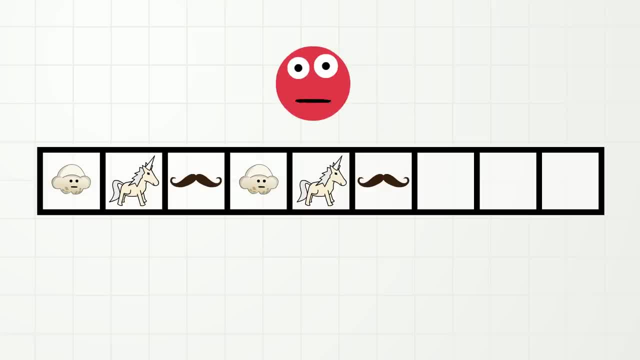 Question number two: What do you think would happen if the pattern keeps going? Do you think it would stay the same or be different? That's right, it would stay the same. The pattern would be the same before and after watch. ah. 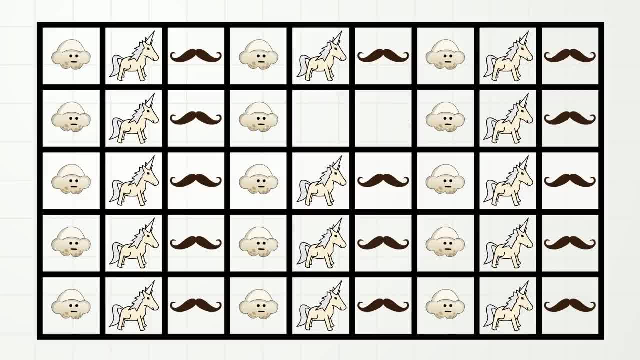 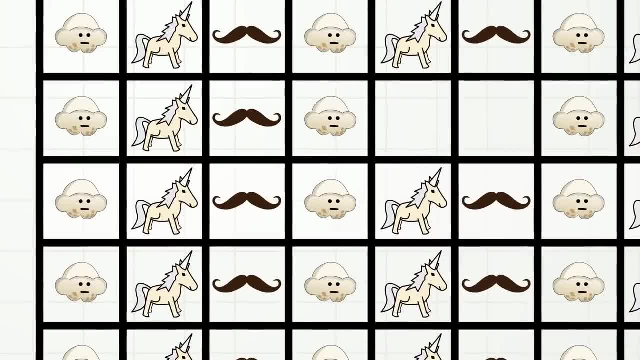 And last question: Oh oh no, some of the pattern is missing. Can you help me fill it in? Let's look. just before the missing spaces There is popcorn, unicorn moustache, then popcorn, So here popcorn. 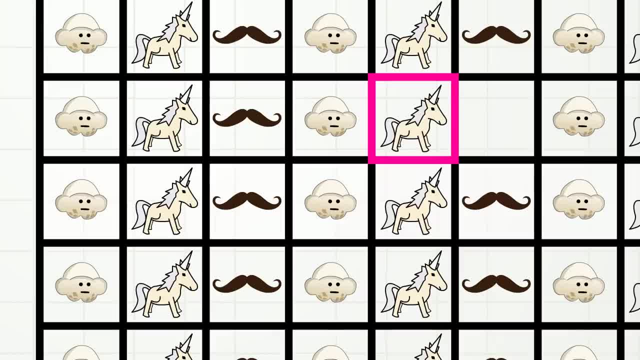 Would be what? That's right, unicorn, And let's try to figure out the last space. So there is popcorn unicorn moustache, popcorn unicorn orange juice. No, let's try again. Okay, popcorn unicorn moustache.